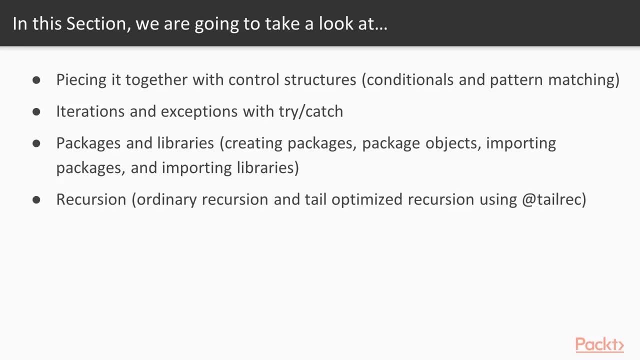 and we'll focus on the package object. Finally, we'll be doing recursion. We'll be looking at the conditionals and pattern matching, Then we'll be doing iterations and we'll see that tile recursion is an optimized version of the ordinary one. And this is the first. 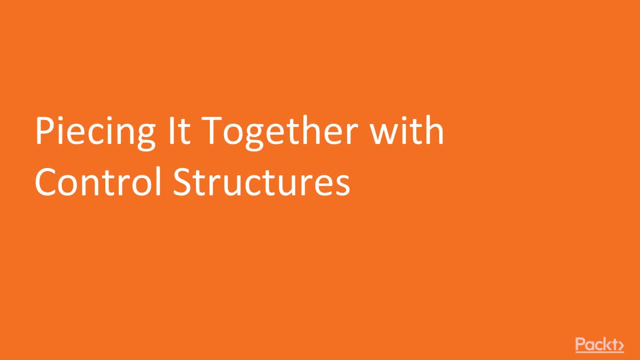 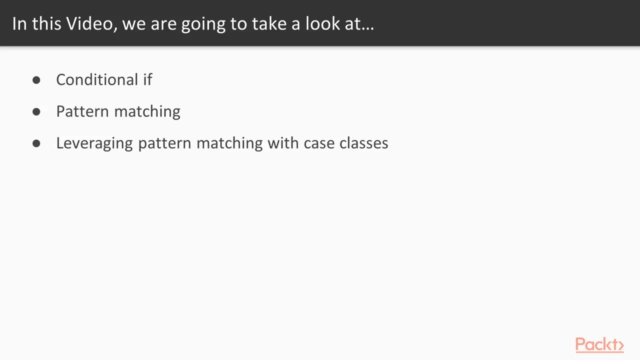 video in which we'll be piecing together our logic with control structures. So we'll be looking at the conditional if we'll be doing pattern matching and we'll be leveraging pattern matching with case classes. So let's start from the simple case So we can see that we should use simple. 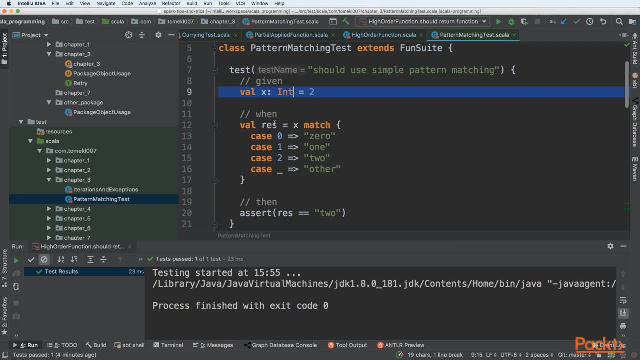 pattern matching. So we are creating an x and assigning 2 to it, And then we are using the match keyword. This is a very important keyword in Scala and every functional programming. So here we are matching. So if the x is k0, so it means if it is equal to 0, then you are just returning 0. 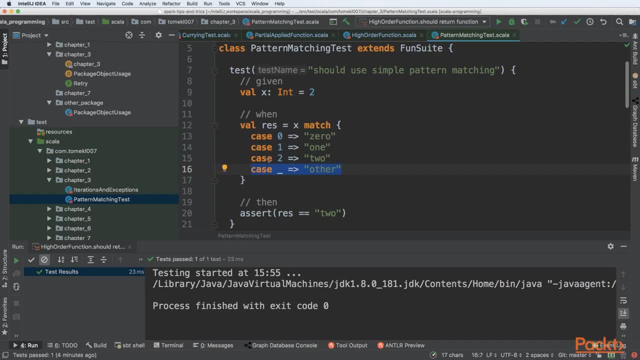 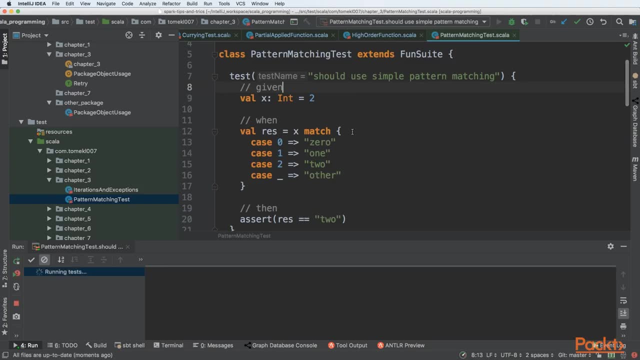 Otherwise 1, 2.. And if it is other than 0,, 1, 2, we are just returning other. So let's start the test and see that the result is equal to 2.. You can right now have an impression. 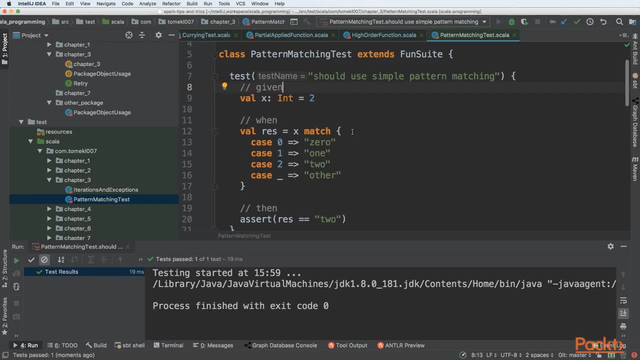 that this is very similar to the switch statement, but pattern matching is way more powerful. For example, we can see that the result is equal to 2.. So we can see that the result is equal to 2.. So we can see that the result is equal to 2.. So we can see that the result is equal to 2.. 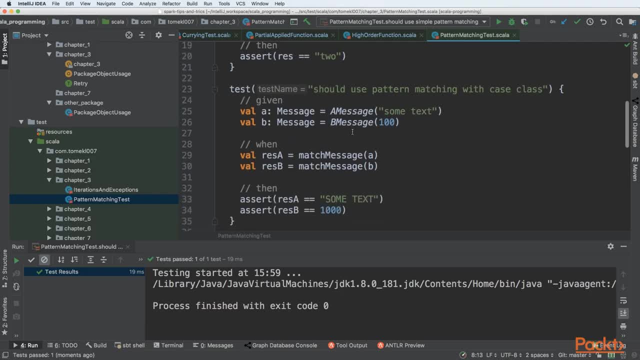 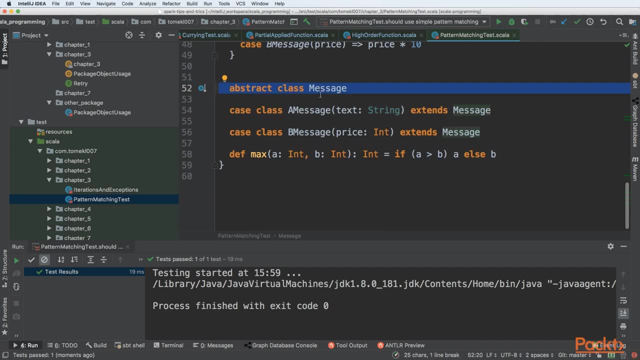 For example, it allows you to decompose your case classes. What does it mean? Let's take a look. So we are creating an hierarchy of classes, We are creating a message that is an abstract class, A message that just extends message and gives a text, and B message that has a price. So we can. 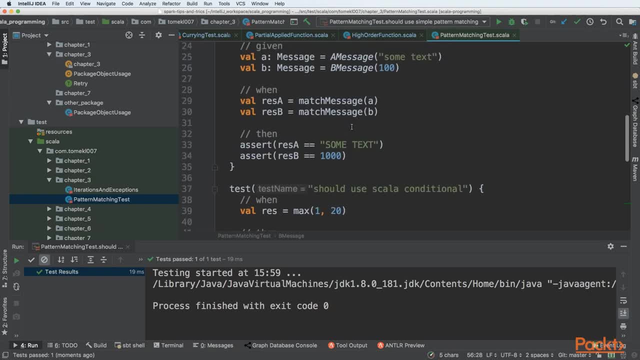 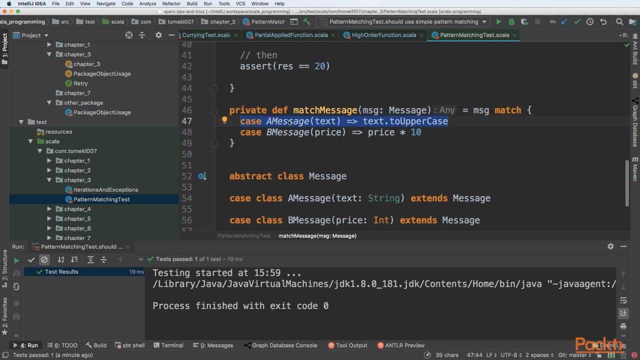 see that both of those messages has different types of fields. Then we have a match message method that is matching those messages. So we can see that if the message is an A message, then we are taking 2.. So if the message is an A message, then we are taking 2.. 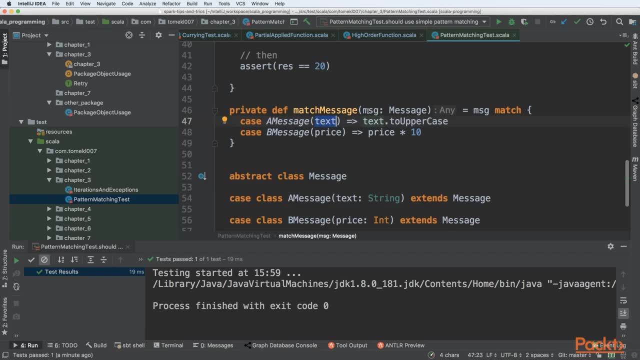 a text and that text will be extracted from the message. and here we have an access to the text we can do to uppercase and it will just return this type. if it will add b message, then the price will be extracted and we are multiplying it by 10. we can see that it will return to any. so if 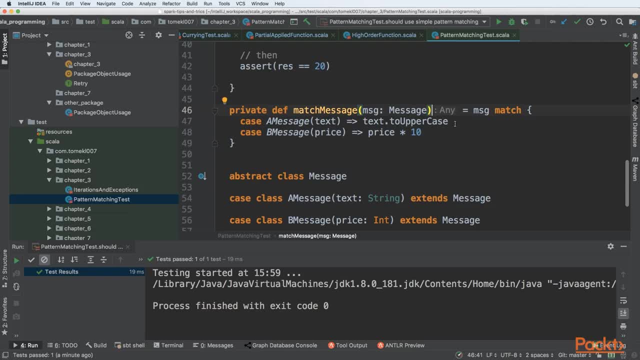 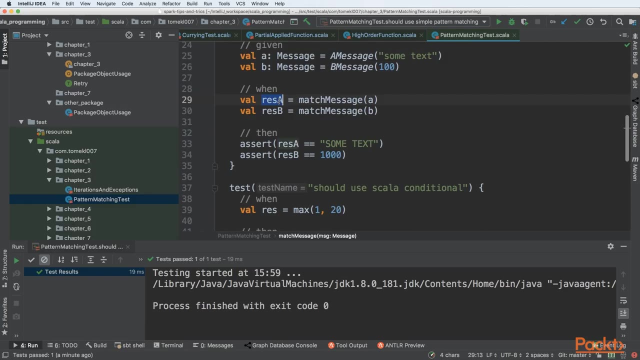 you remember from the first section about hierarchy of inheritance. in scala, any is a subtype of anything. it cannot be anything different because here we are returning string, here we are returning the integer. so one common type is any. so at the return we have a result a and result b. we can see: